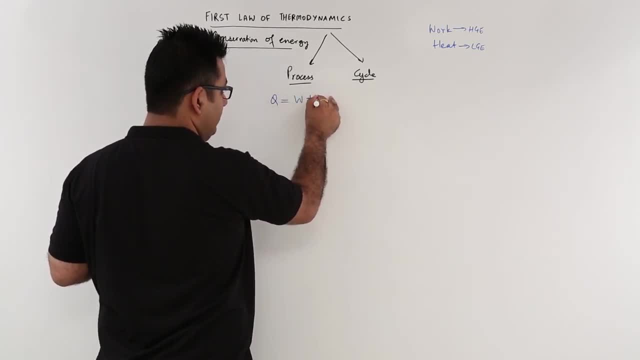 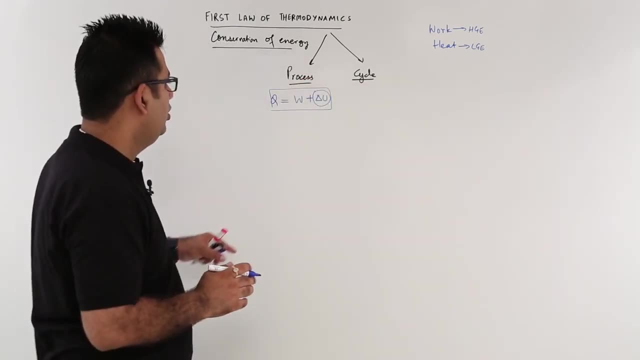 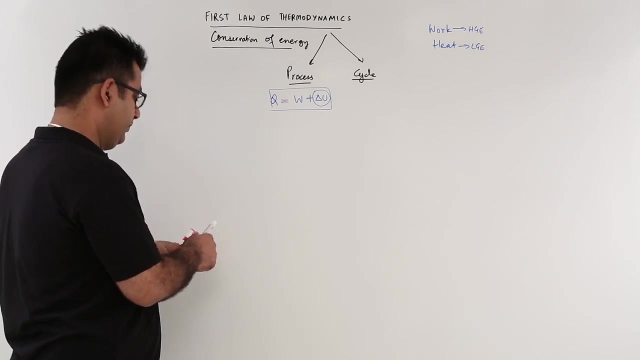 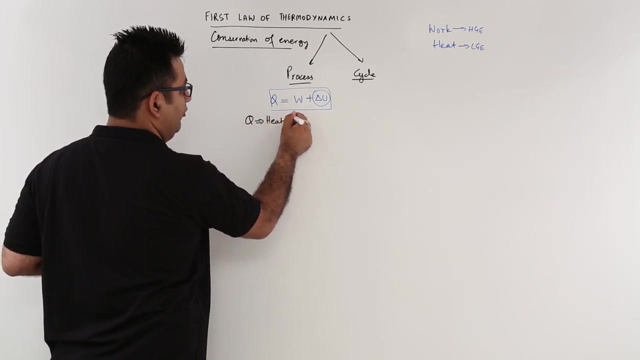 It gets converted into work. plus, some of that heat is utilized to increase the internal energy of the system. So this is the mathematical relation for the first law for a process, Okay, where the value of Q- This is the heat flow Okay- To or from the system- depends. 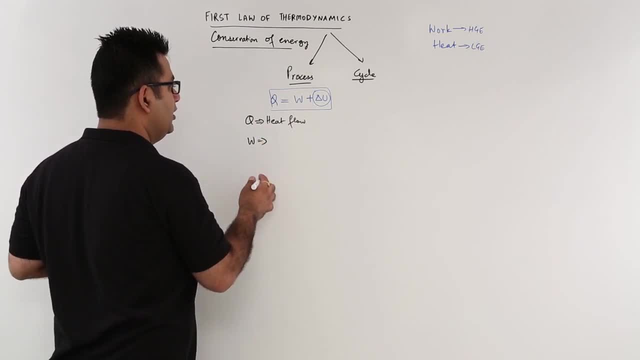 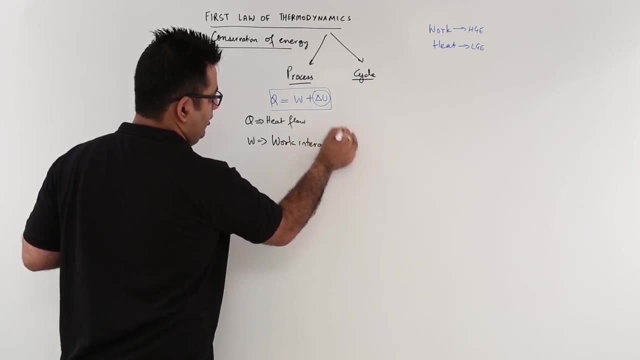 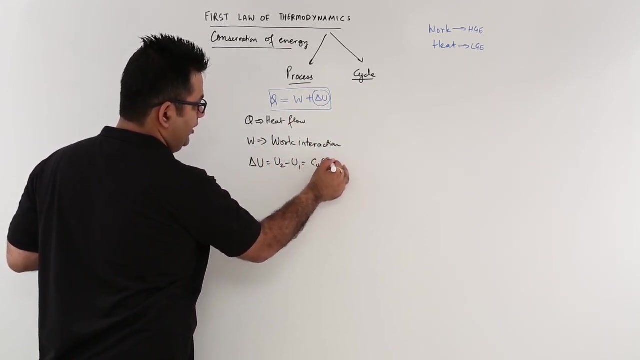 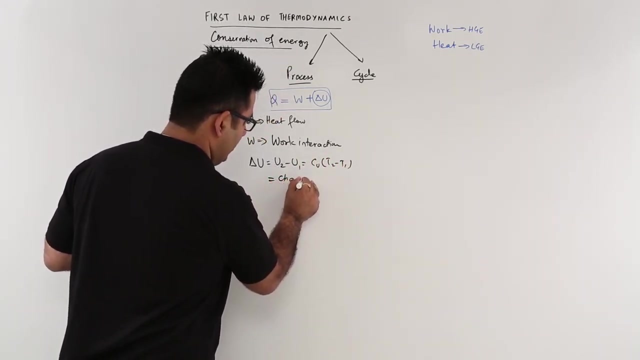 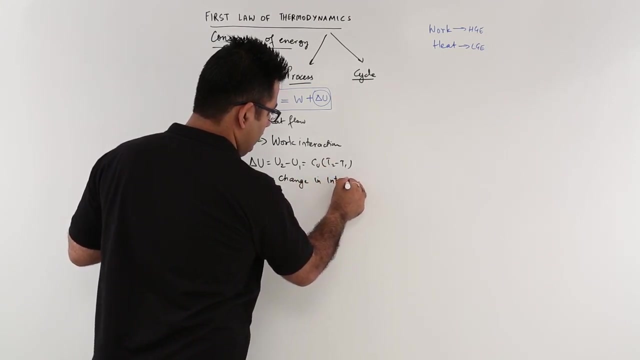 will have the you know relevant sign convention for that. So W is the work interaction, ok, and delta U, which is U2 minus U1 or Cv into T2 minus T1. ok, This is the change. I would not say increase or decrease, just change, ok. Change in the internal energy of the system. 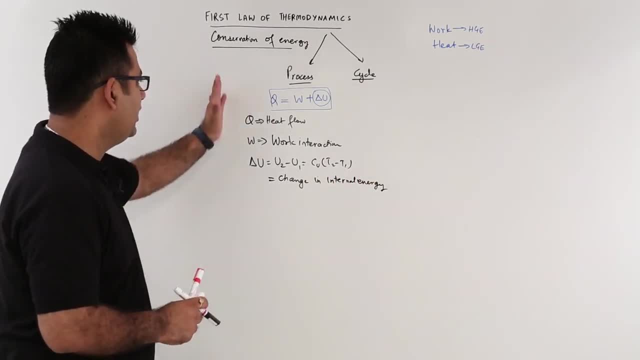 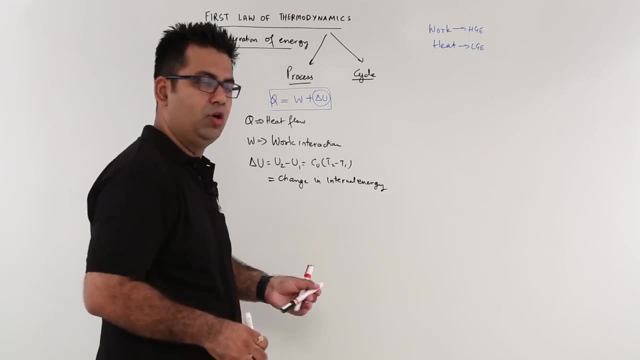 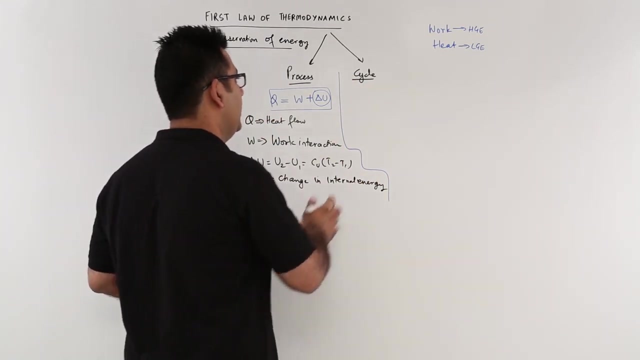 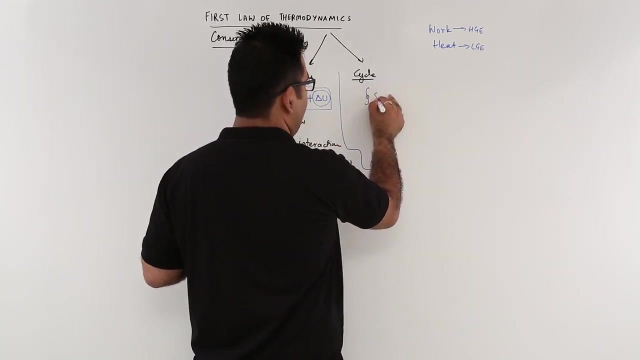 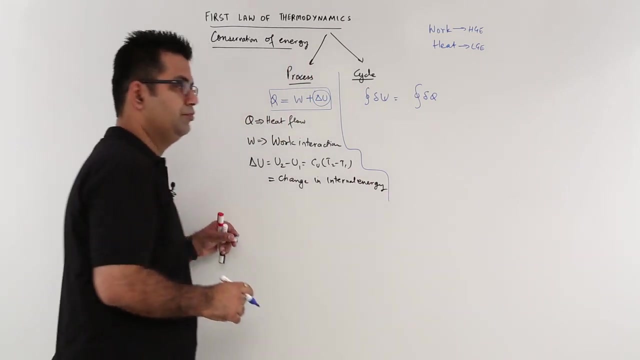 ok, So that is the mathematical relation for a first law for a process. ok. Now, if you talk about the first law applicable for a cycle, the first law application for a cycle, ok, Then this becomes integral or cyclic integral. ok, Delta W: this is equal to cyclic integral. delta Q. ok, So 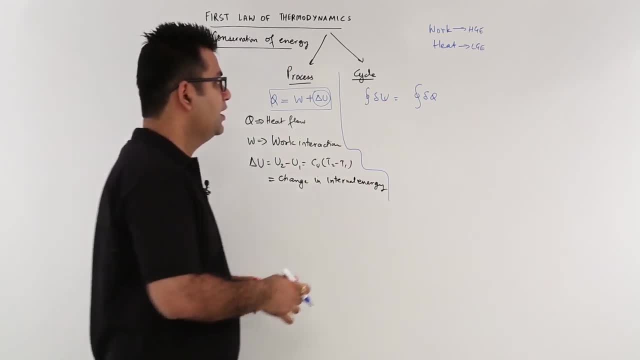 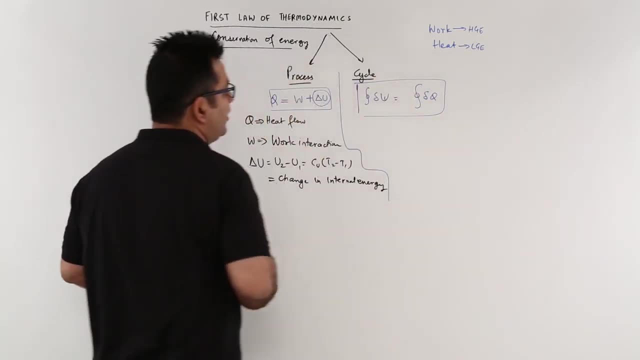 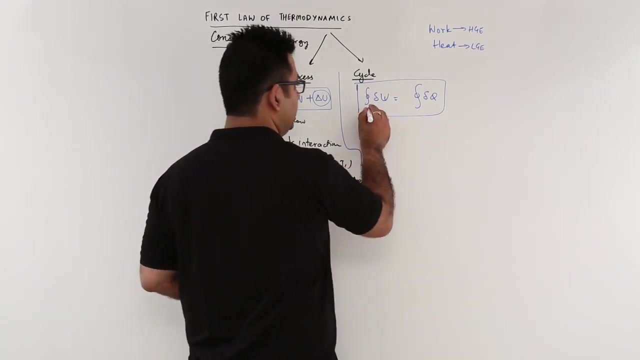 the net work interaction in a cycle is equal to the net heat interaction in the same cycle. ok, So these two are the mathematical relations for the first law, So let me define these values. So this is the net work interaction: the net work interaction during a cycle, during a cycle. 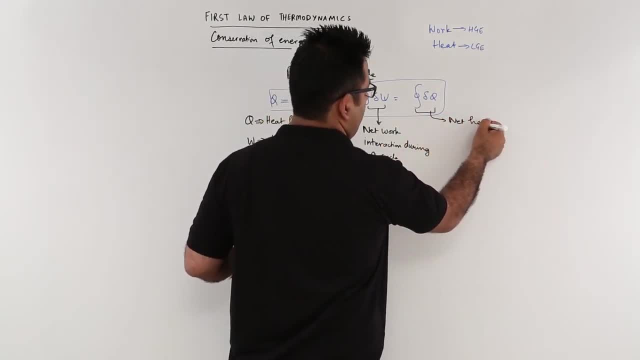 and this is the net heat interaction. net heat interaction during a cycle. ok, Now, for example. so for the next one I am writing, this is the net heat interaction, niin D and so on, and so on. Bien, is that ok? Nimочка d x, dp. theBuilding a fire school. Now, in terms of the frPC Frein.